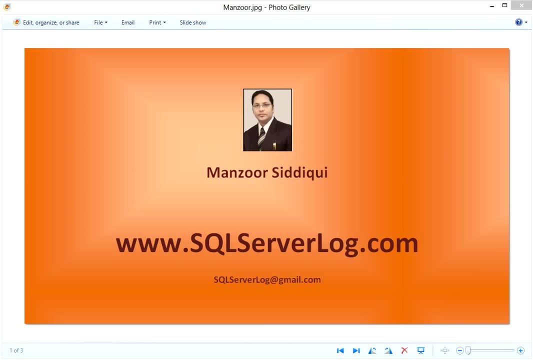 Encryption is the process of protecting data with key or password from unauthorized access, so that if data is stolen or hacked, then also it is safe and secure. Today we'll see how we can protect our valuable data and database with transparent data encryption feature available with SQL Server database. 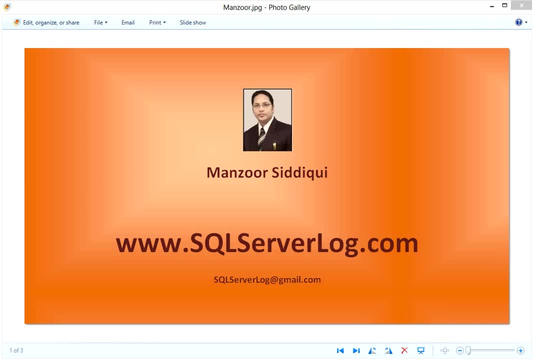 As a database administrator, you take database backups regularly and keep the backup copies on a storage drive or tape. If those files are stolen or somebody tries to misuse data by restoring it, then how will you protect it from cracking or decrypting? To handle such situation, we use transparent data encryption. 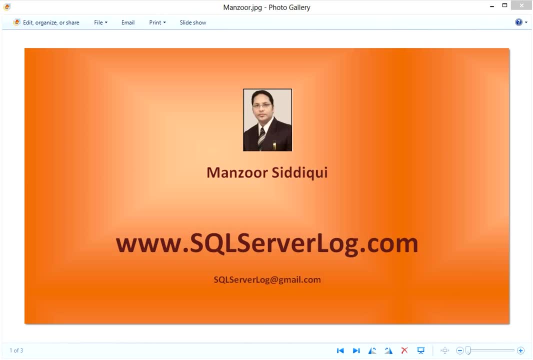 So, basically, in transparent data encryption it uses database encryption key, which is also called DEC, which is secured by certificate and kept in master database. Database encryption key is either protected by certificate or an asymmetric key secured by extensible key management handler with the help of Microsoft cryptographic API. 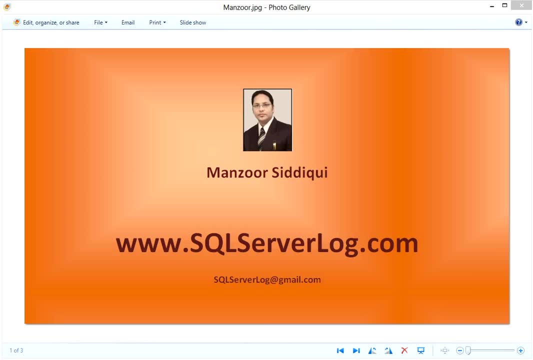 In TDE, data is encrypted using Advanced Encryption, Standard and Triple Data Encryption, Standard encryption algorithms. Transparent data encryption technique is used at database level. Database encrypts it before writing And it is decrypted at the time of reading. Hence you can observe IO encryption and decrypting of data file and log file. 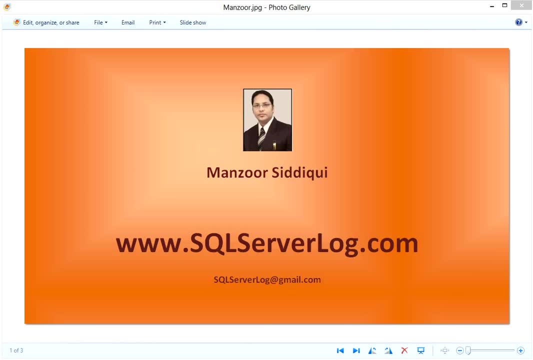 Also, you may face performance decrypt, because if you are using any database encryption on database instance level with TDE, then TemDB database will be encrypted automatically. So when you back up a database without encryption, you'll be able to read beauty's table. 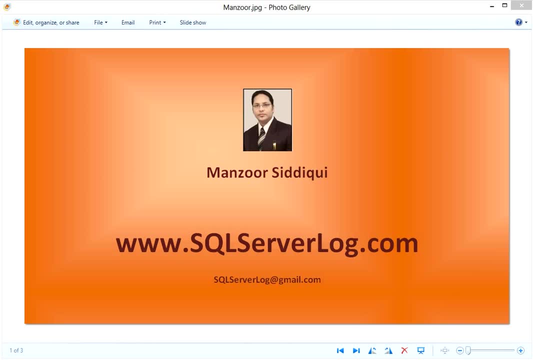 content. i will show you you. you will be able to read its content row by row, and our main motto is to encrypt those readable contents inside backup and log files. so let's go to our database. i'll show you. we have a client info database in sql server 2012 enterprise edition. for demonstration: 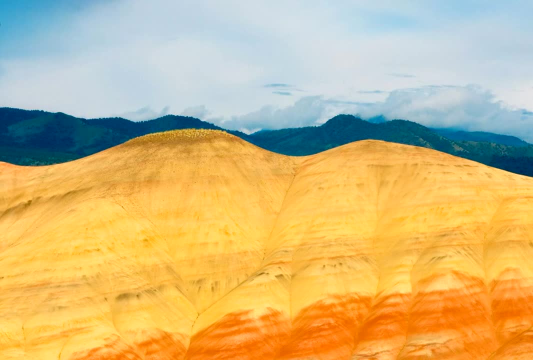 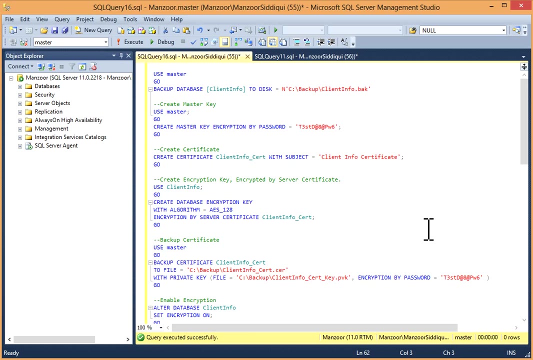 so this is my first instance. i have written all the queries here, so that will follow step by step process to encrypt the database and will restore it on other instance. this is my default instance, mansoor, and right now i'll just refresh my database. so i have. 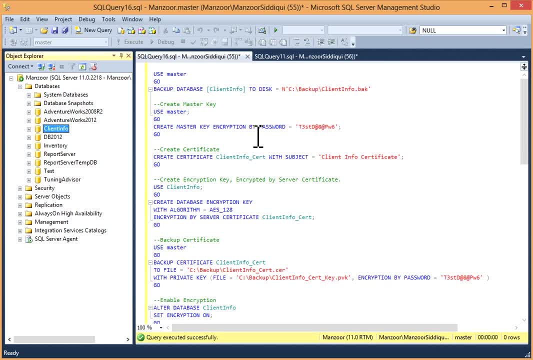 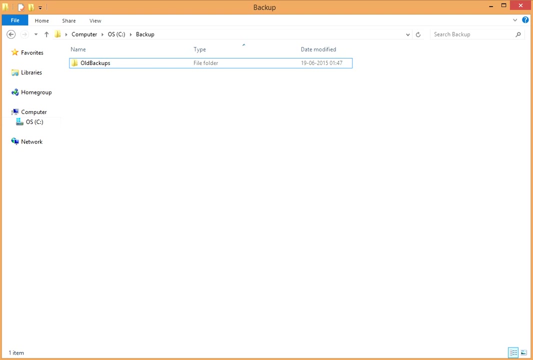 client info database. okay, which we will encrypt. so first of all i'll show you data inside database. suppose, for example, if you are taking backup, normal backup, this database is right now not encrypted, so i'm taking this backup on c drive backup folder. so in c drive backup folder, this is my c drive backup folder. no backup file is available, right? 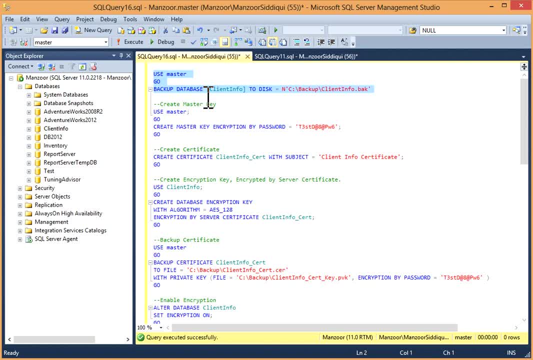 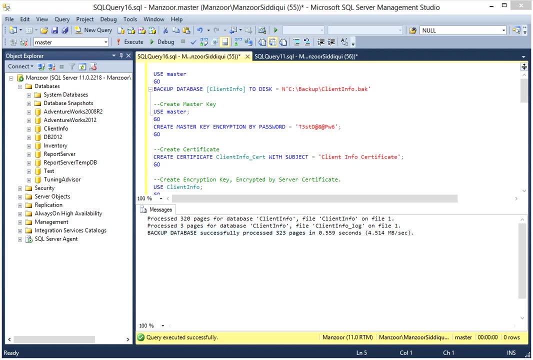 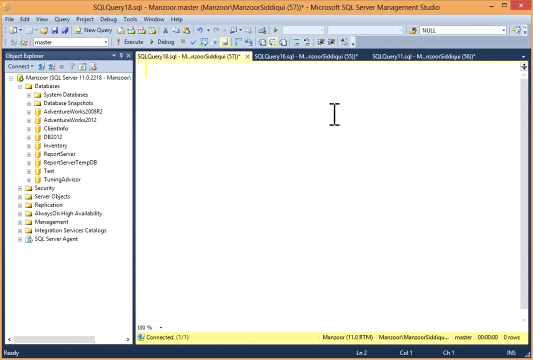 now. now i'm taking backup, selecting backup database, client info to disk c drive backup folder: client info dot bak. execute backup database successfully processed. so this backup file is created. now we'll go to our backup file. i have a table inside this client info database, so one table is vendor, so i will select. start from. 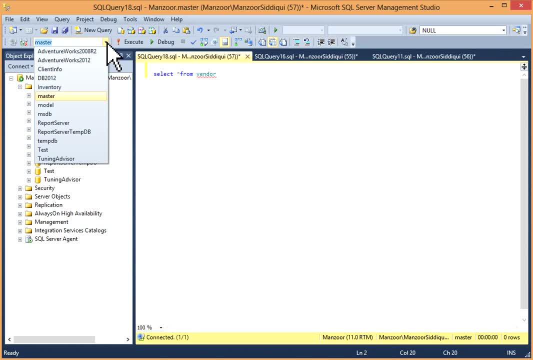 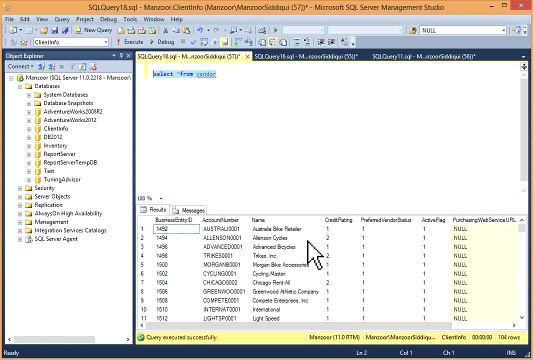 vendor and i will select database client info and execute. now you can see business entity id, account number, name and other details are available, so i'll just take any account number. for example. first one: australi 0001. this is australia bike retailer, so i'll just copy it. now i will show you exactly what is happening. 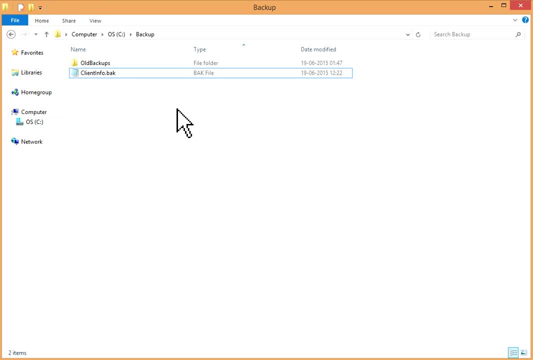 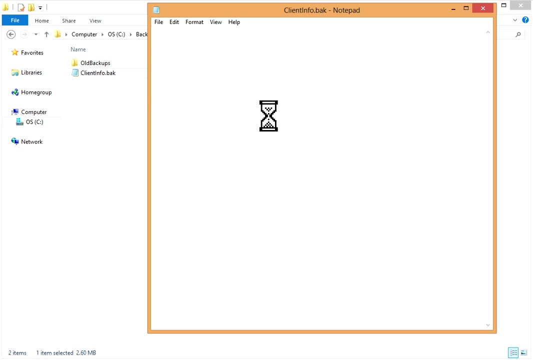 behind backup up now. this is your backup file. if you'll go right click on it and open with any editor, I will just open it with notepad so you will be able to find those records. yes, you will be able to find those records. so this is this. data is not secured. this is at this take. this is 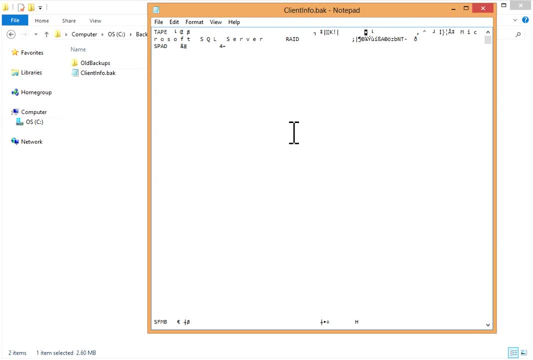 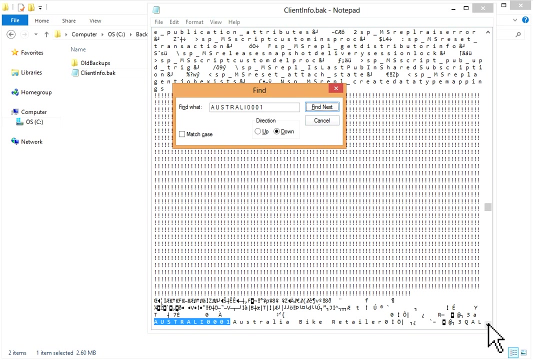 taking some time. yeah, so now we have backup file details. I'll just search it. this is my account number for Australia bike retailer. this data in backup file is stored like this, so I will search it and and you are able to find it. this is Australia triple. 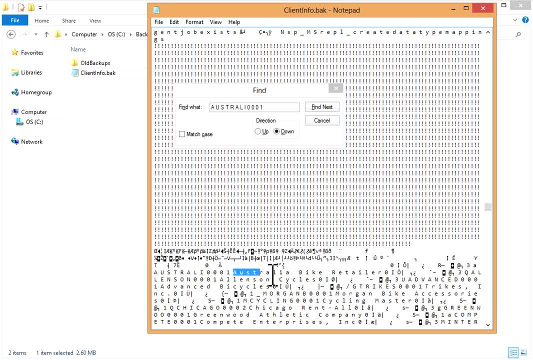 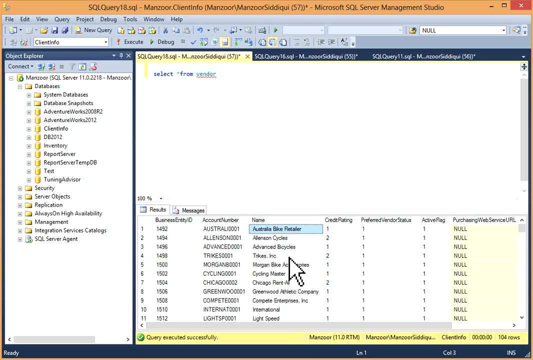 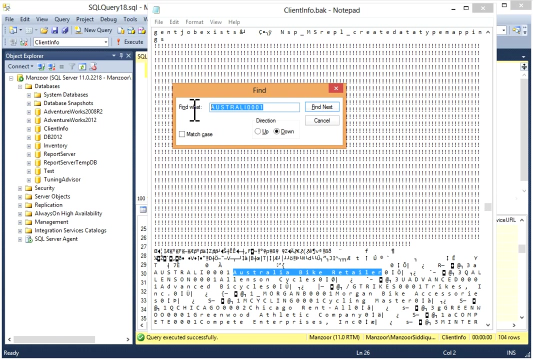 zero, one account number you have found, then, who the name is: Australia bike retailer, like that. if you are searching any other account number, for example this one, I will just take any other example, for example, Hills bicycle service. this is account number now find you are able to find it. okay, account number, name and other data, you are eligible. 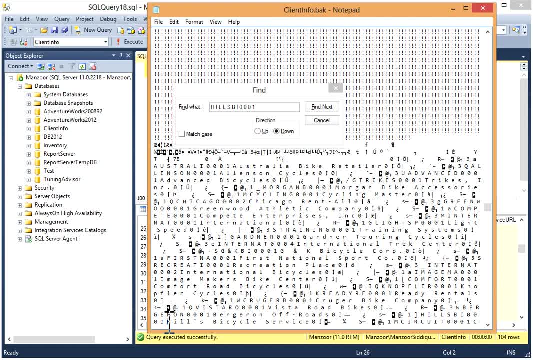 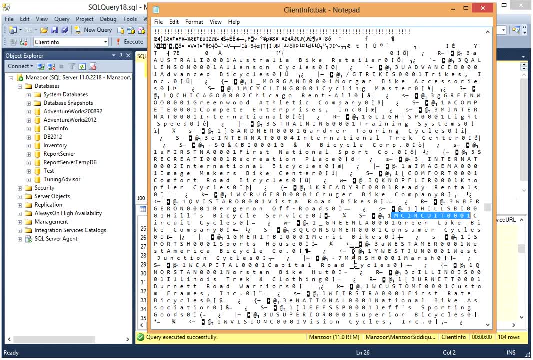 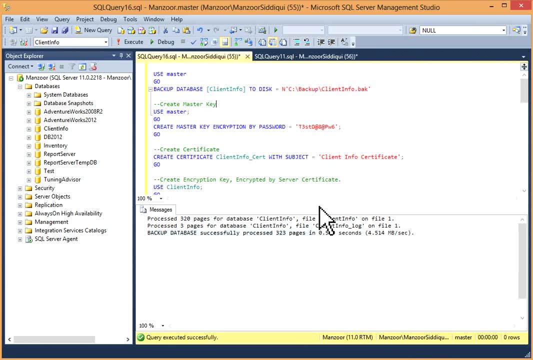 to find it okay. account number, name and other details are available. so so our main motto is, main purpose is to encrypt this data. i'll just close it now. we'll return to our step. we have taken normal backup. now we'll create a master key. in this process of tde, you have to 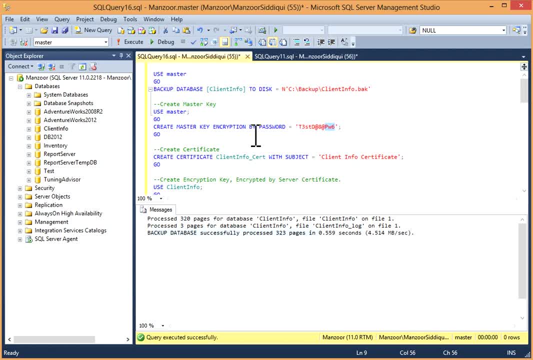 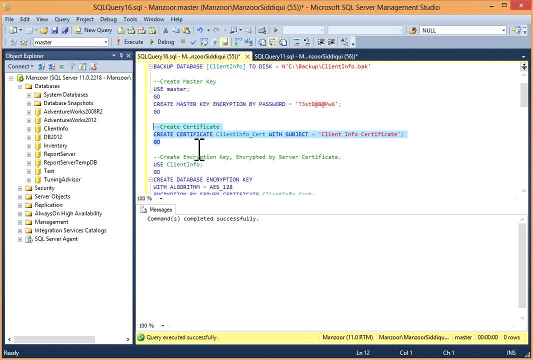 create a master key encryption by some strong password. so this is the syntax: create master key. encryption by password equals to a strong password. execute master key we have created. now you have to create certificate. so create certificate. client info underscores that i have given this certificate name with subject. you can give your subject details. 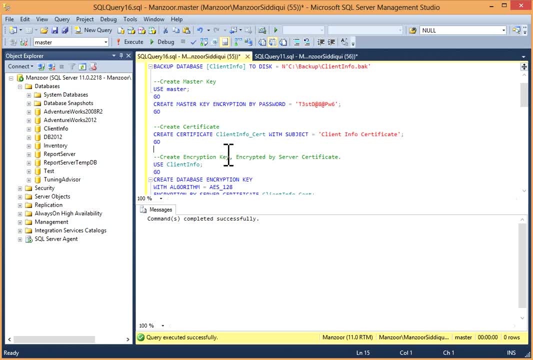 select it and execute. certificate is curated. okay, now create encryption key encrypted by server certificate. now you have to use this: create database encryption key with algorithm: advanced encryption, standard algorithm, aes encryption by server certificate. we are encrypting it by certificate, this one which we have created. client. 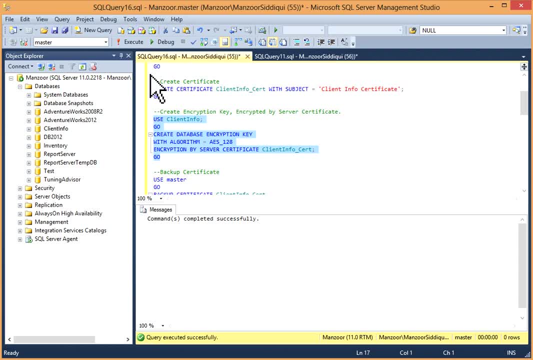 for underscore set. okay, so i'll just select it and execute: see the warning. the certificate used for encrypting the database encryption key has not been backed up. okay, you should immediately backup the certificate and the private key associate with the certificate if the certificate ever becomes unavailable or if 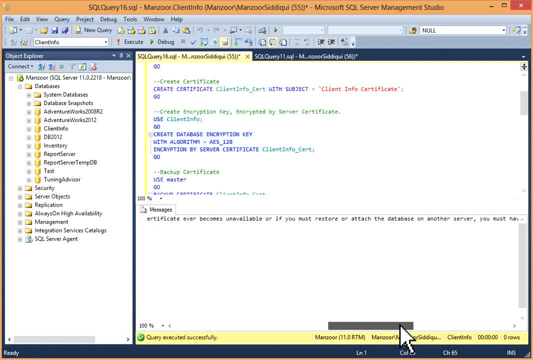 you must restore or attach it, attach the database on other server. you must have backups of both the certificate and the private key or will not be able to open the database. so it is very important to have both certificate and private key so as per instruction will take backup of certificate. so backup certificate your. 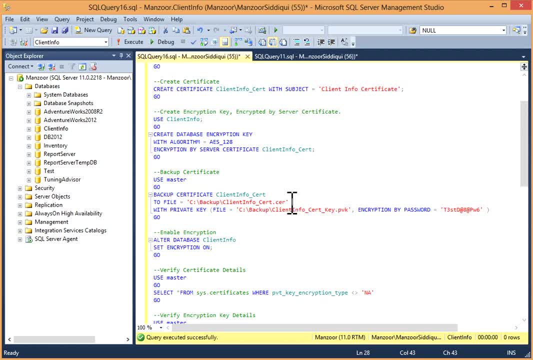 certificate name to file. okay, so we are creating this file on this path- backup path- and certificate name is client info, underscore set dot CR, C, ER and with private key file equals to C drive backup. I'm creating this private key on the same location. encryption by password: this password is our master key password. 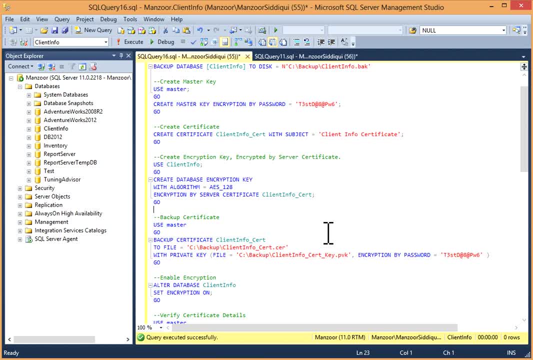 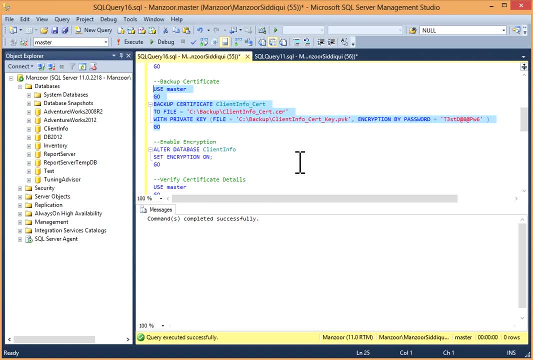 as we have seen earlier. this one, so I'll just execute it: successfully created. now we have to enable it. you have to enable encryption. alter database: database name is client info. set encryption on execute. now we have created certificate, we have created encryption key and I just want to show you how to do that. so we have created a certificate, we have created encryption key and I just want to. 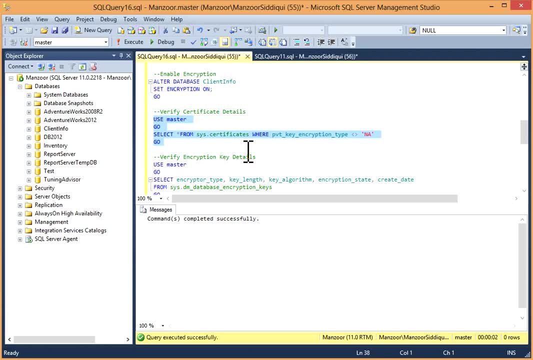 verify it, so I'll write. select a start from C start certificate where you can give where condition, if you want. otherwise, no problem. select a start from sister certificates. execute it now. you can see you have created client info underscore cert. okay, this is a certificate ID. this is master key. 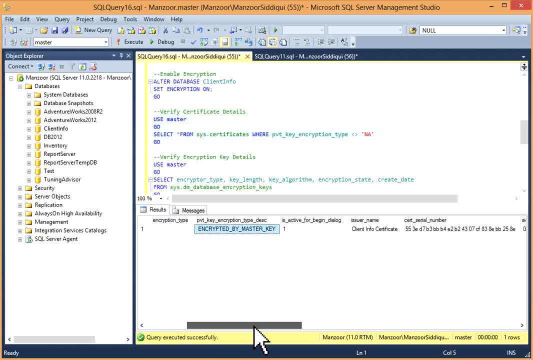 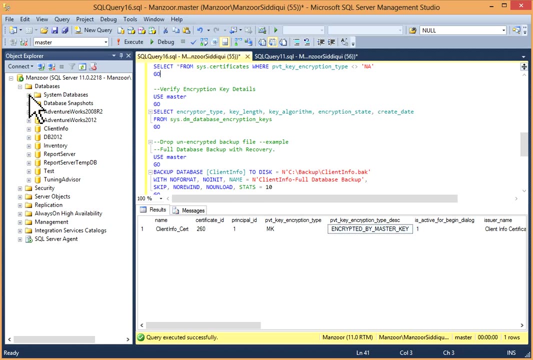 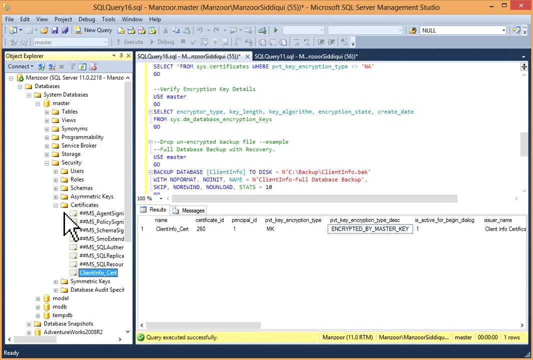 encrypted by master key. okay, this is issuer name: client info certificate and all these details are available here. now you can also verify because this research in system database, master database. I will show you this certificate. I'll just refresh it: master security certificate. this is a client info underscore cert, so we have verify. 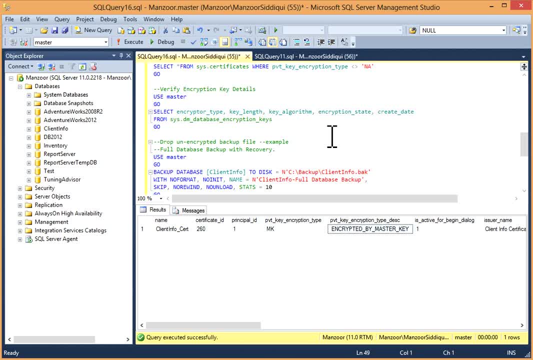 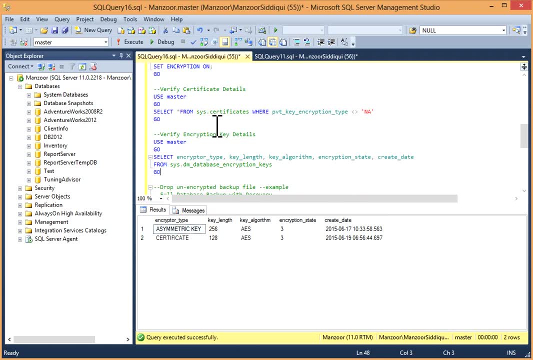 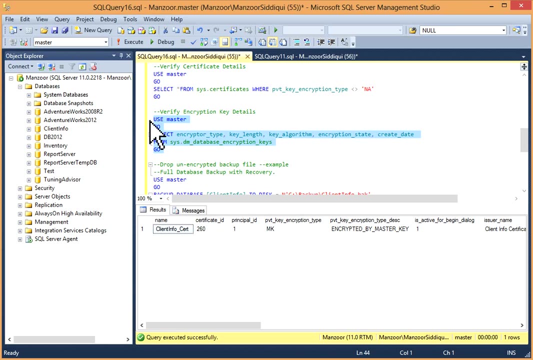 it. we have checked this one. no, okay, we have checked this one certificate. now verify encryption key details: encryption: encryption state is 3, so encryption is on this asymmetry key and certificate key length: 256 and 128 AES. advanced system, advanced standard algorithm. advanced encryption standard algorithm. and now we have taken. 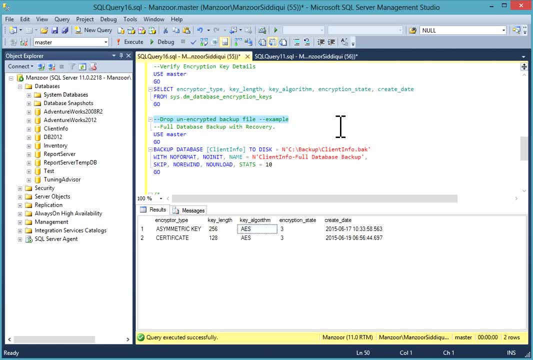 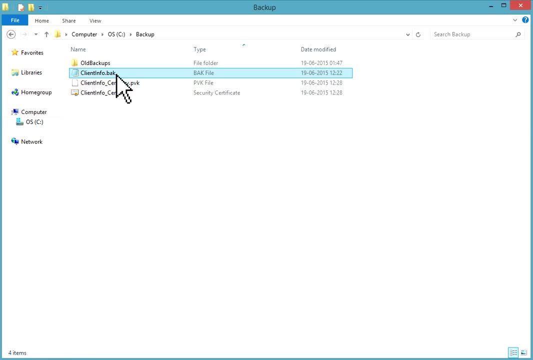 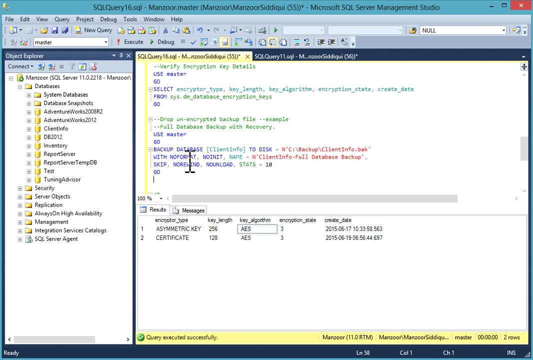 one backup file, for example, which I have shown. so that was unencrypted, so I'll first go and drop that database backup file. I'll just delete it now. I'll take database backup backup database database name to disk equals to backup client info: dot back. okay, I'll take backup now. just remember that this. 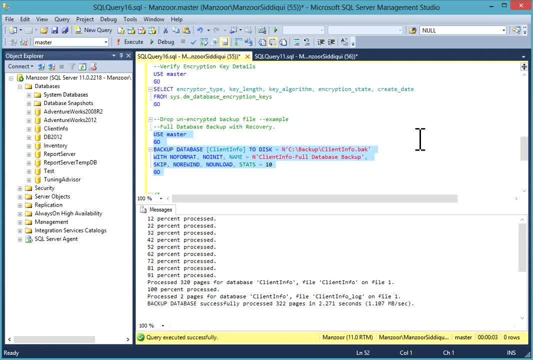 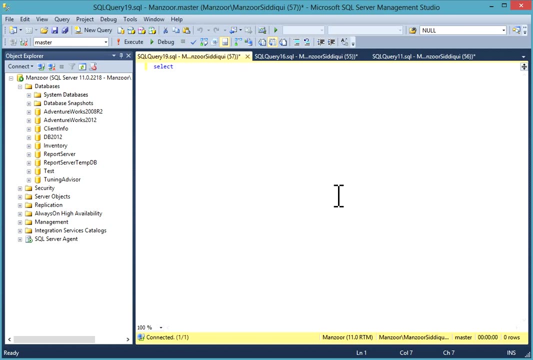 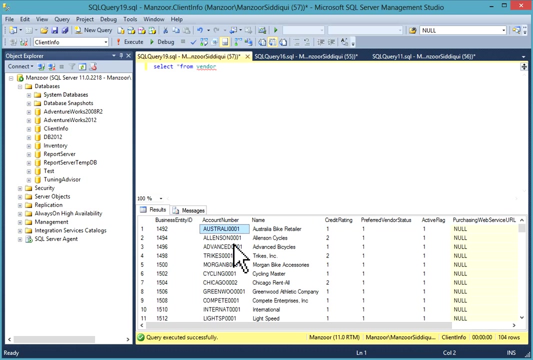 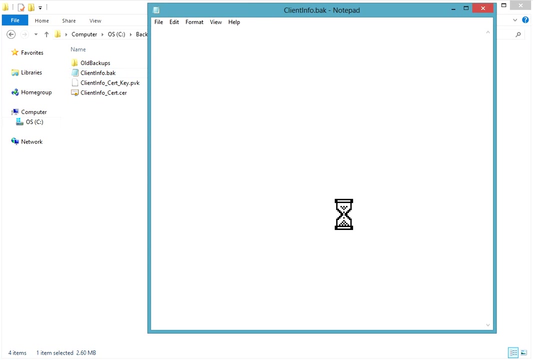 is our encrypted database backup. now this backup database successfully processed again. again, Nobody have encrypted Backup file. and across check select he start from Bender. okay, in client info database again I'll take same account number and we'll go to our Clinton Force database back up file I look on with. 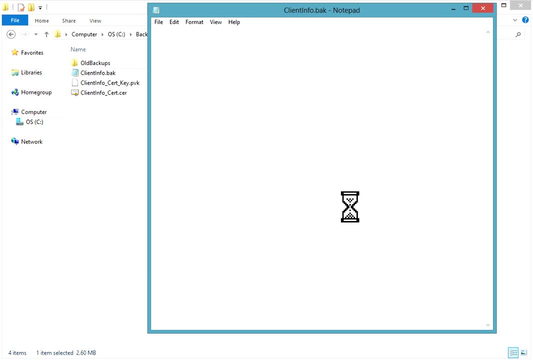 editor notepad. we'll again try to search that record- account number and name. we are just cross-checking whether this is really encrypted or not. so if the record is available, it will be able to find it. if it is not available, you won't find it. so 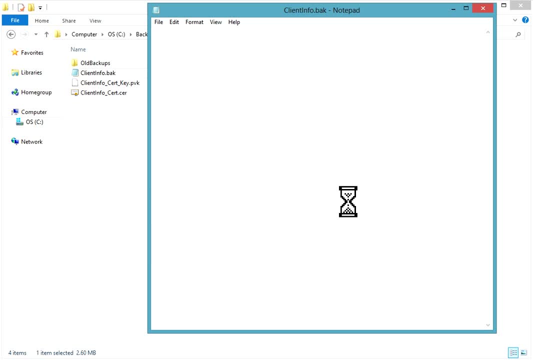 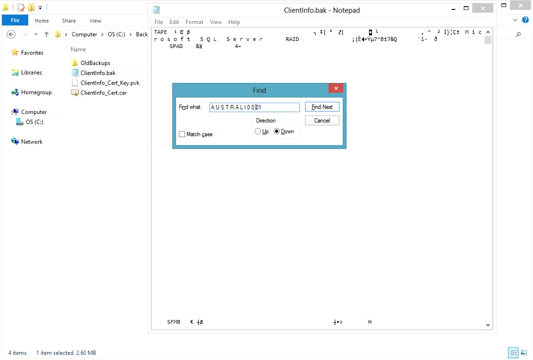 right now and this is loading. once it is loaded, we'll search it. as you can see, this certificate we have created. client info cert underscore key- dot. pvk and client info underscore cert- dot. CR certificate and master key we have created. so now our database backup file is open. now we'll try to search it. see, cannot find this cannot. 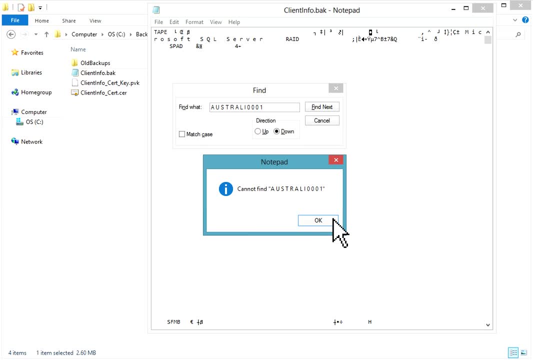 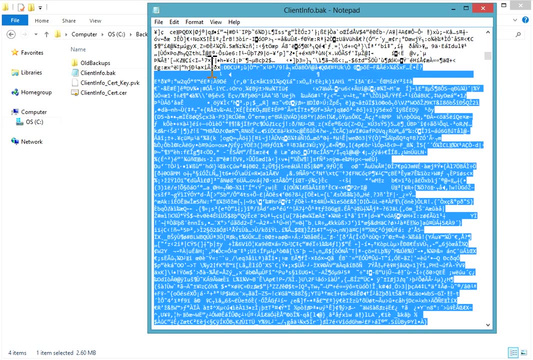 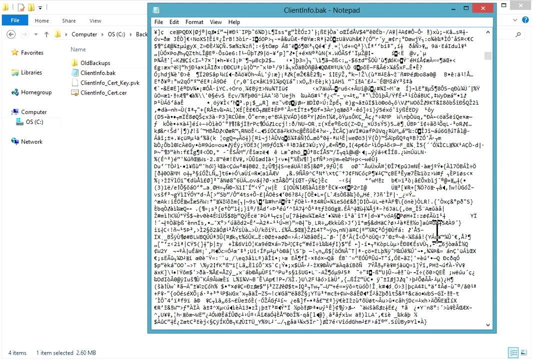 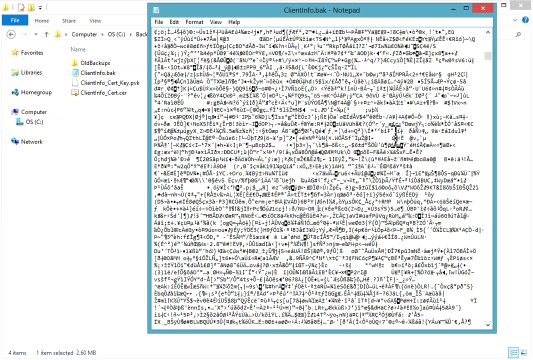 find account number. so your data base backup file is encrypted. now, if we will go here now see, see the encryption, just see the symbols. earlier it was readable, some part was readable and some critical information were available. right now you can't read it. okay, so this is now encrypted file. 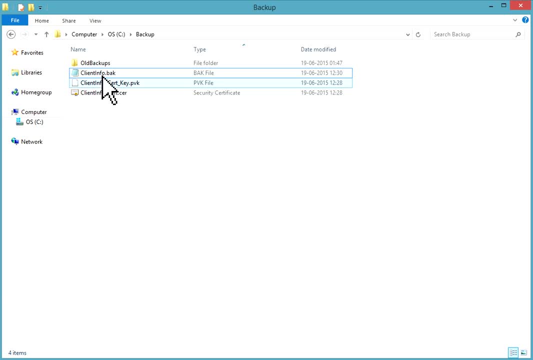 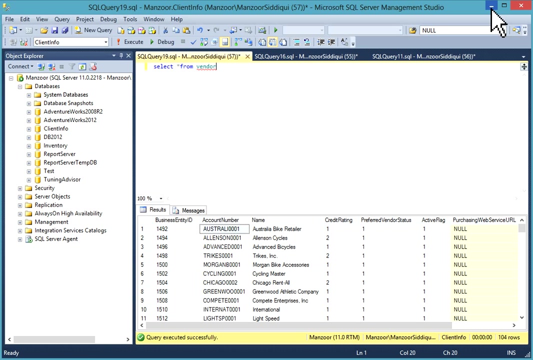 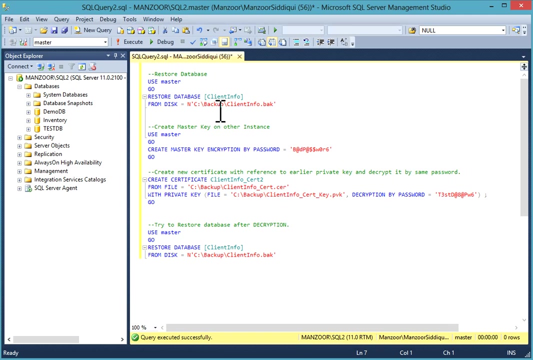 now the same database, client info dot BAK. if we will restore, suppose, for example, somebody has stolen it and he is trying to restore on his instance. okay, so we'll go to other instance. this is my other instance will too, and I have this query. I will try to restore this database and just see the message this. 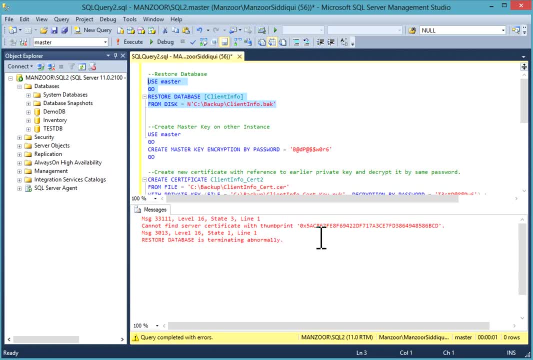 is executing cannot find server certificate with thumbprint. this one it is stored. database is terminating abnormally okay, so you are not able to restore this database. if somebody has stolen it or you have misplaced your file and somebody is trying to see some records from backup file, he is not able to do. 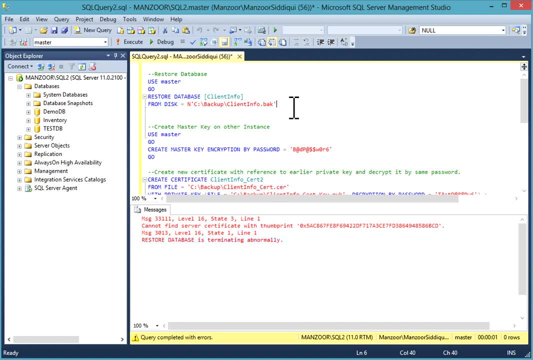 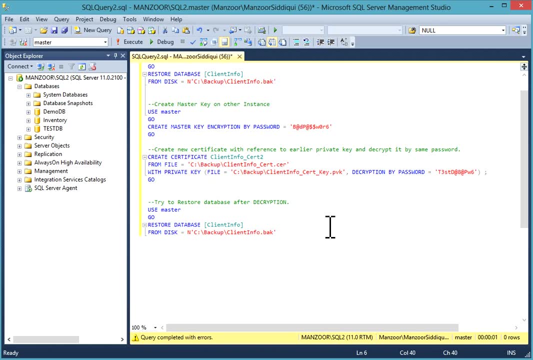 that restore database is terminating abnormally, okay. so again, if you want to restore on other instance, there are some process you should know. you should know that. you should know that. you should know that you should know your master key- okay, your decryption by password and your certificate and your. 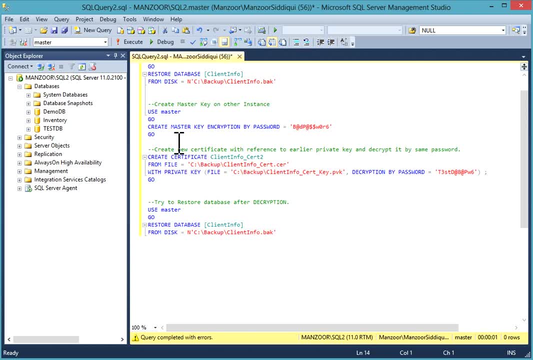 private key you need. so first of all. on other instance, you have to create a master key, encryption by password you have to give. you are creating different master key because this is different instance and you have to specify different password. so I'll just select it and execute it. 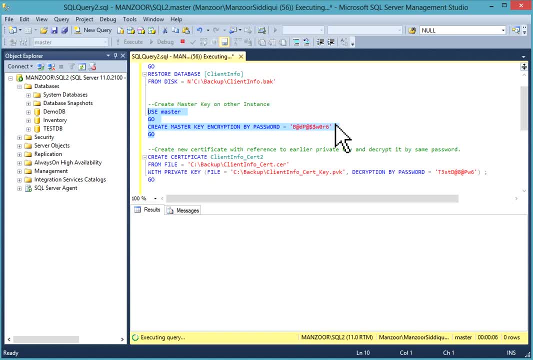 so this is creating master key encryption by password. I have given some strong password. now you have to create a new certificate with reference to earlier private key and decrypted by same password. this is create certificate. you are creating a new certificate. earlier the certificate name was different now because this is my different instance, so you have to create a. 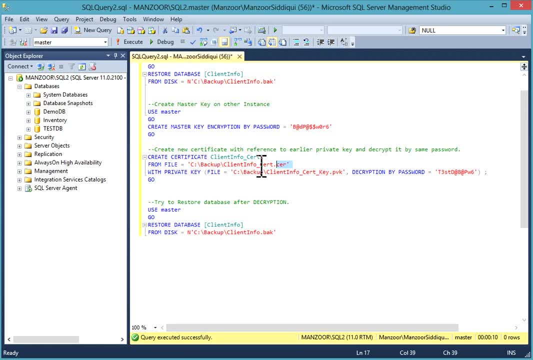 certificate with different name, then from file you are taking the same certificate. okay, which we have backed up this one. okay, we are giving same reference and private key file. this is same private master key and we are using same password. okay, this is decryption by password equal to the, because we have 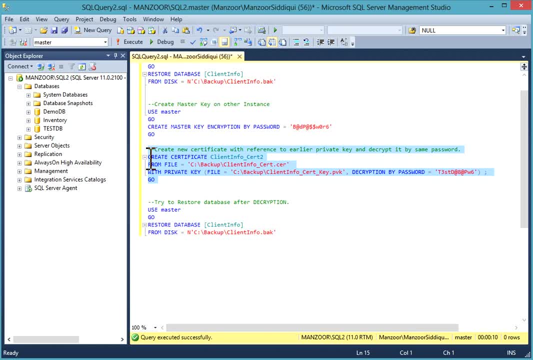 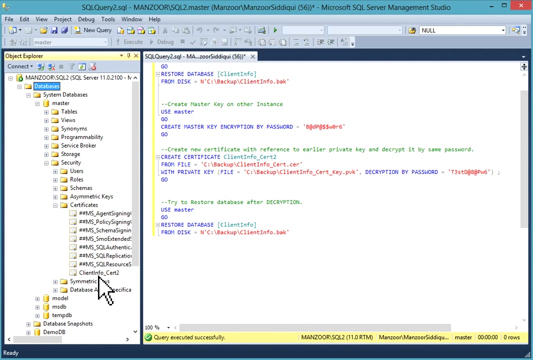 encrypted our backup file with this password. okay, so I will create certificate. certificate is created. now, before certificate is created, I will refresh it and I will show you. go to master security the certificate. now you can seeemen aleg sympan. ok, Now, Again, we will try to restore database because we have decrypted with our password. 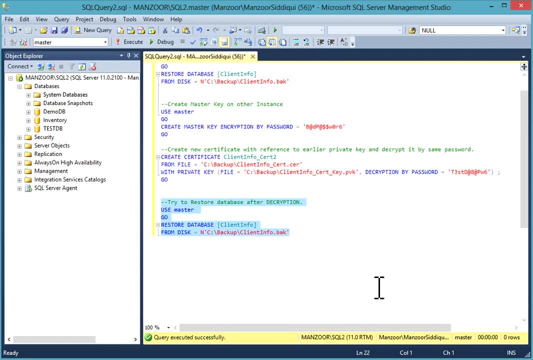 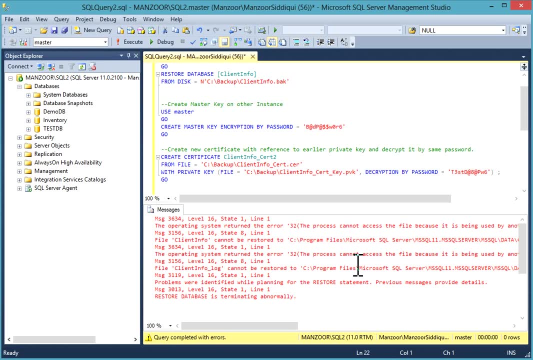 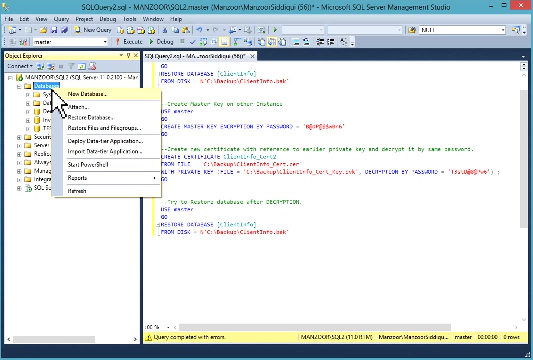 Because I'm genuine user, Okay, so I'll try to restore it. Oops, some problem is there. Yeah, because This is trying to restore on the default path, Default path and there is, I guess, already Database is available, So I'll just restore database with on different path. 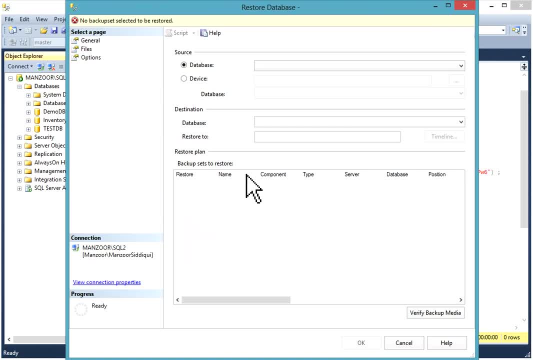 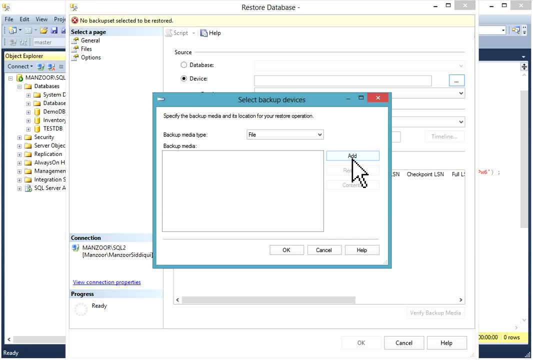 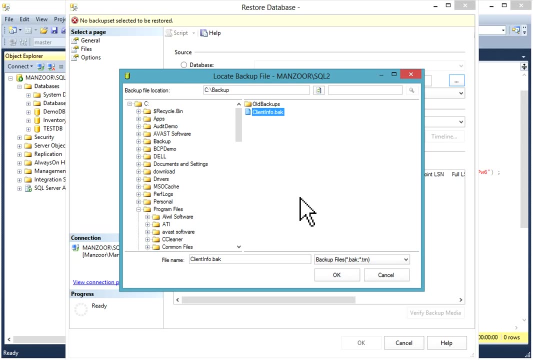 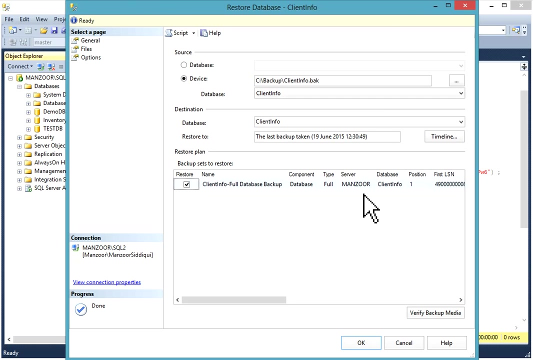 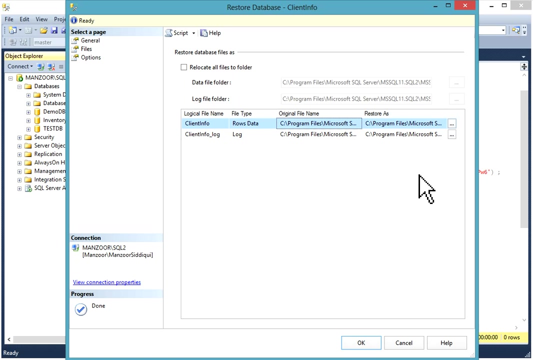 So this is loading Device. Select your path. Add. Go to your backup file. client info. dot back Selected. click OK. Okay, it is selected. go to files. This was because original file location and restore file location was same. That's why it was giving message, So I will just change it.